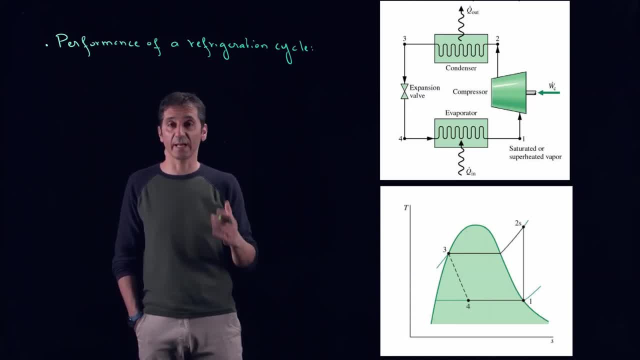 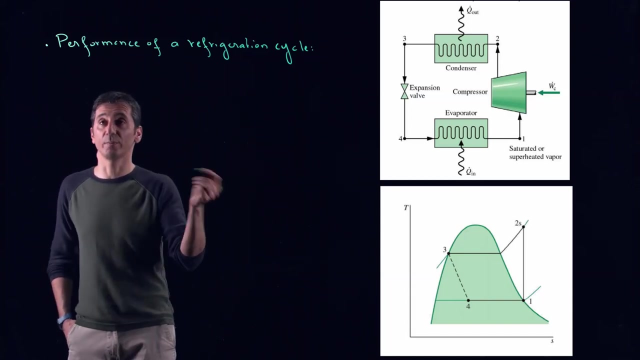 same way. okay, so typically we define efficiency as the power out over Q in, but here the objective is not to generate power. what is the objective? the objective is to cool down, to extract more Q dot L. okay, and what we are paying for this to be done is our work in. so, basically, the 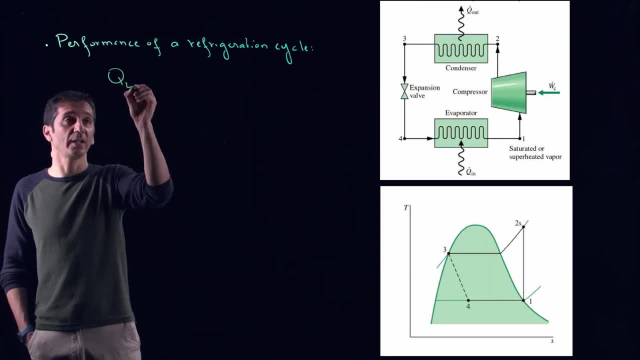 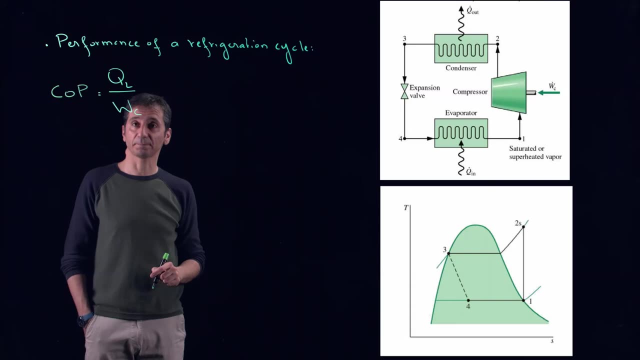 performance is our Q dot L or Q L over the work of the compressor, and we will be calling this it's not an efficiency, will be calling this COP coefficient of performance. okay so, and the first law of thermodynamics is simply telling us that we can write it as Q L over 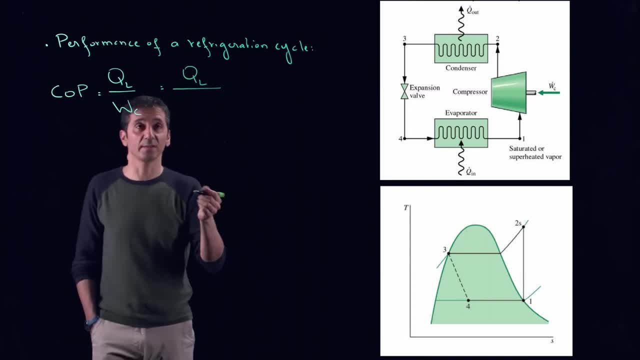 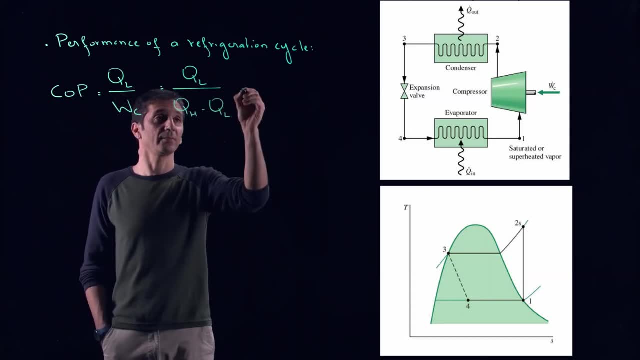 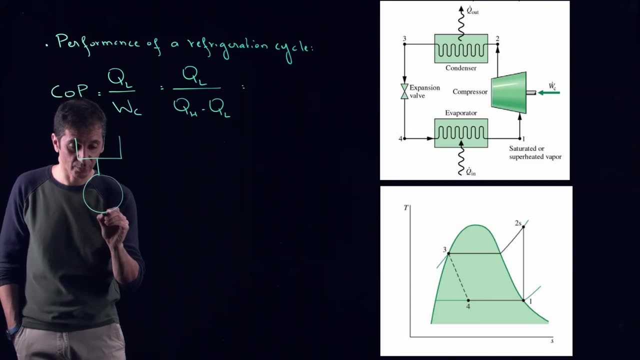 the work of the compressor is equal to what is equal to Q H, what you are rejecting minus Q L. okay, so here you can see it. if I sketch again this cycle or a correspondent, let's say: if I want a kernel cycle, this is TL, this is T H. here we have work in day, we are. 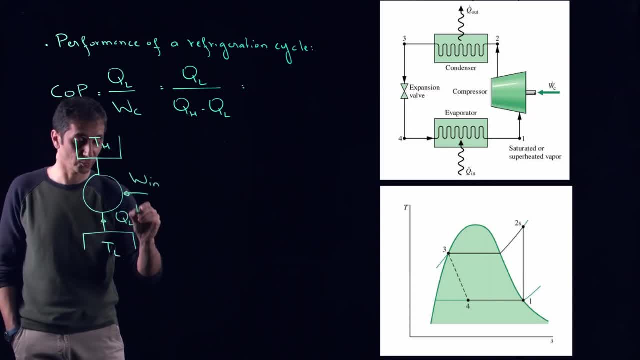 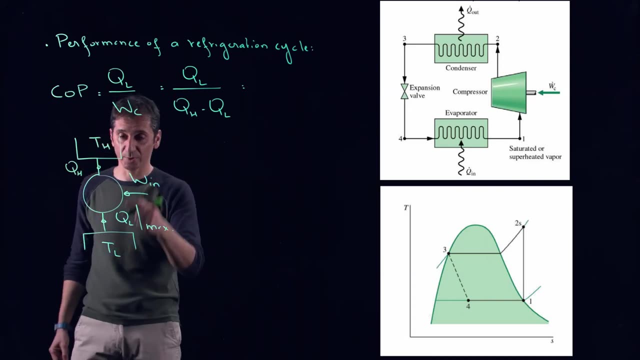 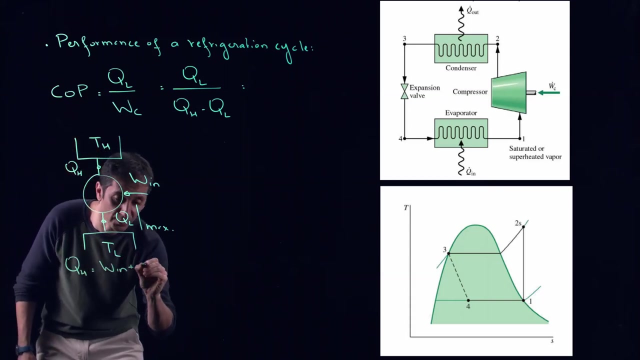 extracting Q L, which is our objective here. this is what we want to maximize and we are rejecting here Q H, okay, and you see that the first law is telling you that the input, the sum of the input, have to be equal to the output. so we have, the output is Q H is equal to work N plus hour, q L and therefore work-in is. 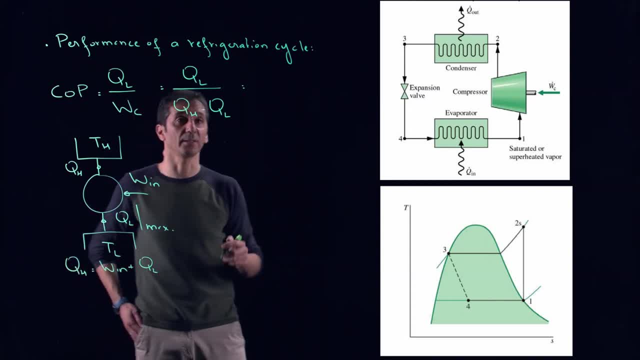 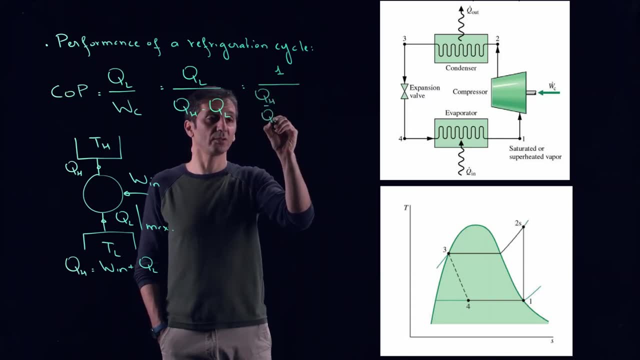 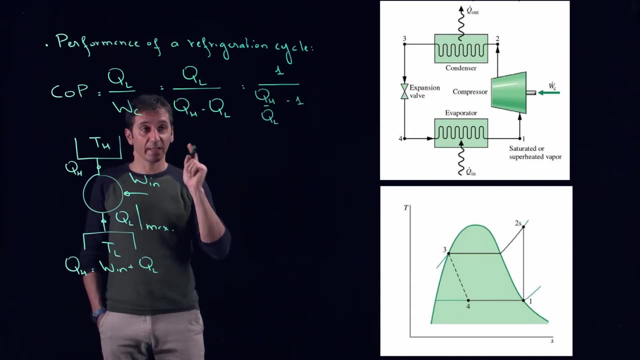 equal to H minus q, H, QL. Okay, so this is what I'm writing here, So then I can write it as 1 over QH, over QL minus 1.. It's only interesting to write it this way if your refrigeration cycle is reversible, Okay.